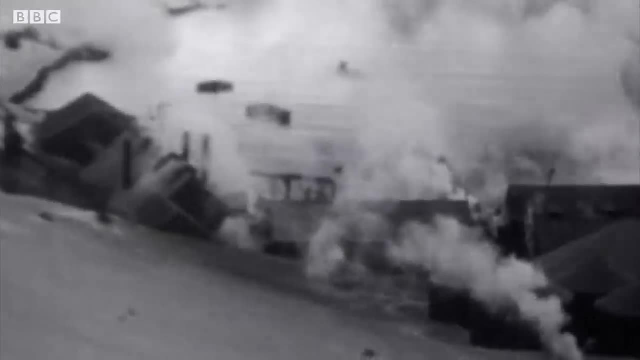 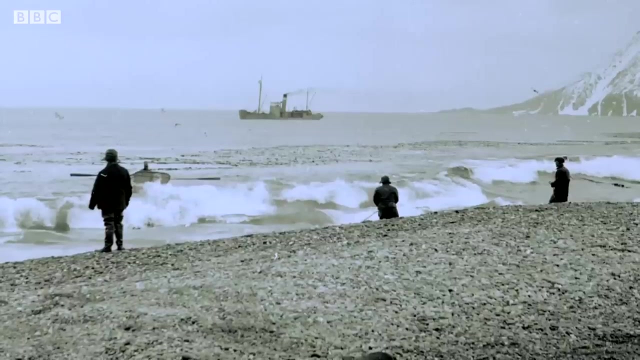 1.2 million were killed for their pelts in South Georgia alone. Seal hunting was the first industry in the Antarctic And from the late 1700s and throughout the 1800s, fur seals on the island of South Georgia were hunted intensively. 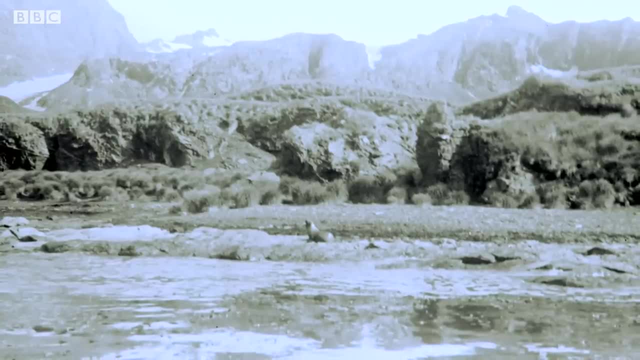 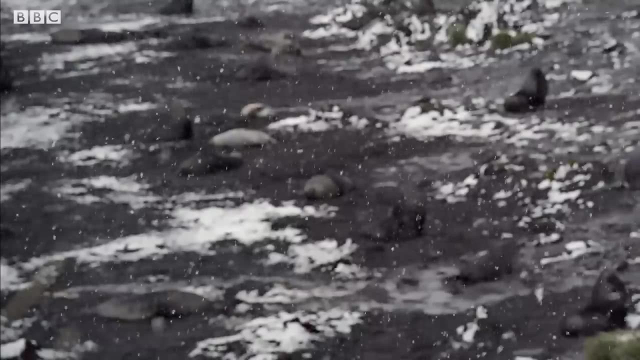 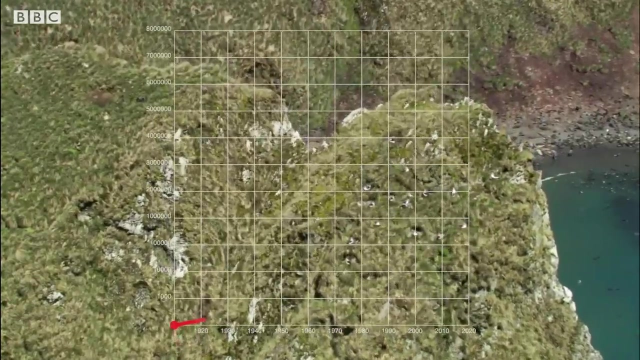 After 30 years fur seals were hard to find. The population plummeted from 1 million to fewer than 400 individuals. By the 1900s fur seals were on the verge of extinction. Remarkably, they bounced back. A small breeding colony was discovered on nearby Bird Island in the 1930s. 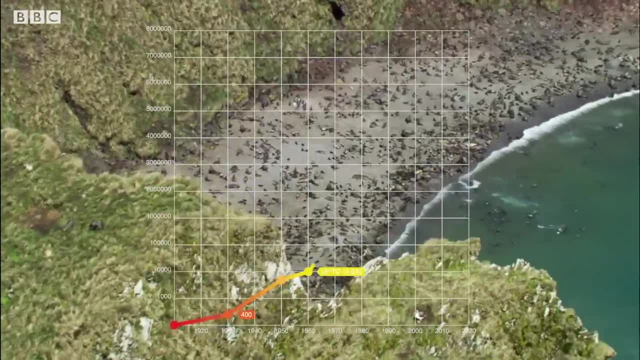 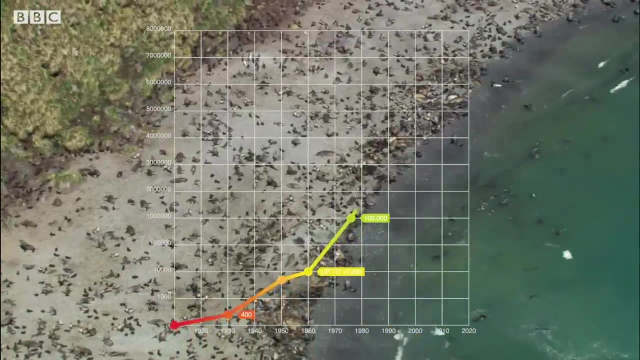 In the 1930s, the fur seals were found on the island of South Georgia. In the 1950s and 60s, up to 10,000 seal pups were being born a year, And by 1976, numbers were thought to have reached 100,000. 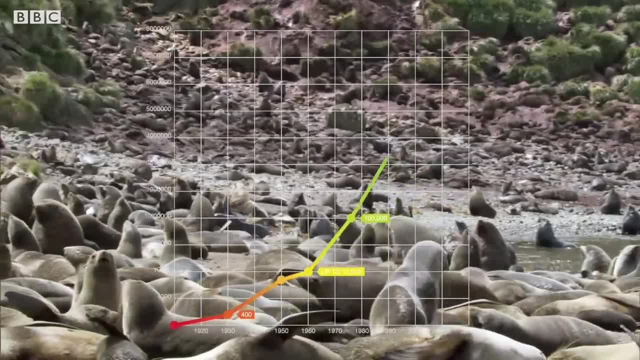 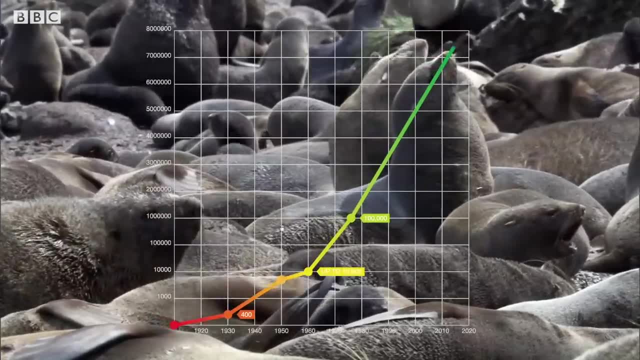 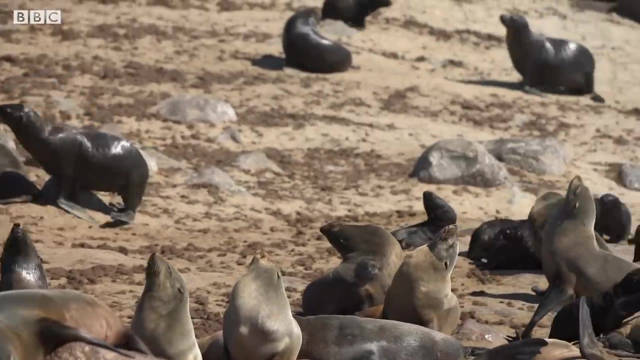 In the 90s, more and more seals were being found further away from South Georgia and its surrounding islands. In 2015,, the population was estimated at between 5 and 7.5 million. 95% of the world's population of Antarctic fur seals now inhabit South Georgia. 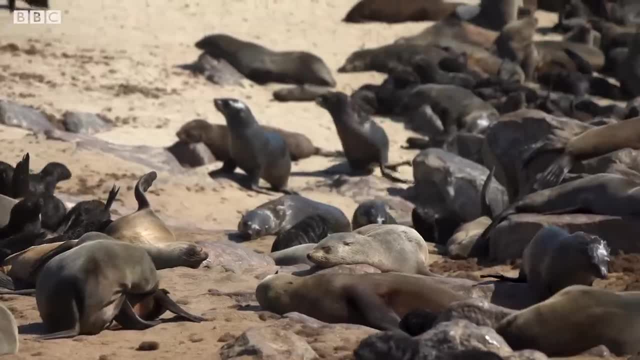 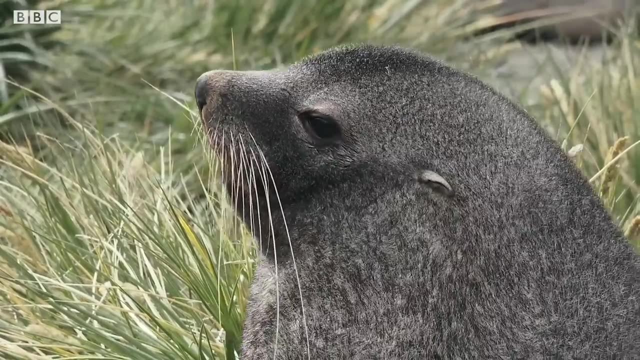 95% of the world's population of Antarctic fur seals now inhabit South Georgia. 95% of the world's population of Antarctic fur seals now inhabit South Georgia. Enjoy the game: Three times the pre-hunting number. An animal the size of a fur seal recovering its population numbers that quickly. 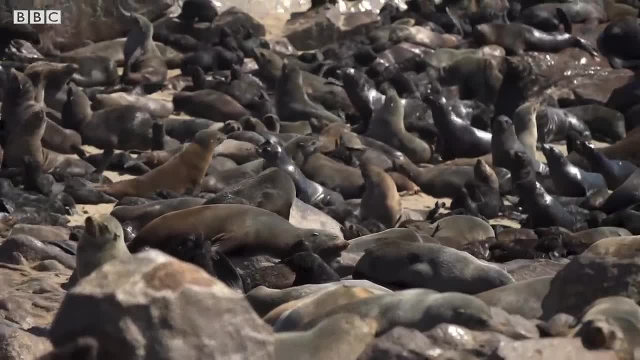 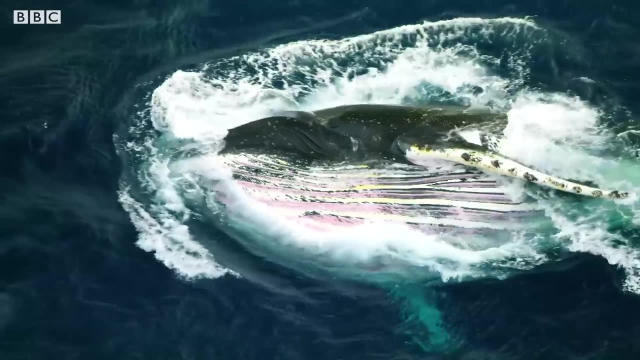 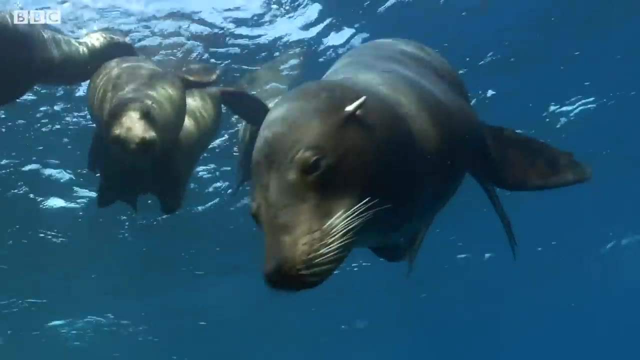 is unprecedented and shows what a remarkable animal this is. So what happened? Seal hunting largely stopped and an increase in whale hunting meant less competition for krill, the seals' main food source. Seals are very efficient predators. They produce an offspring a year. 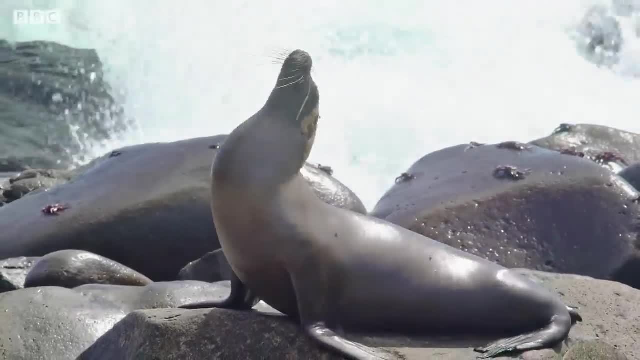 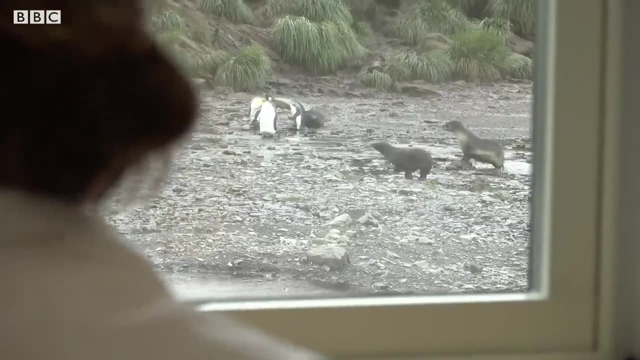 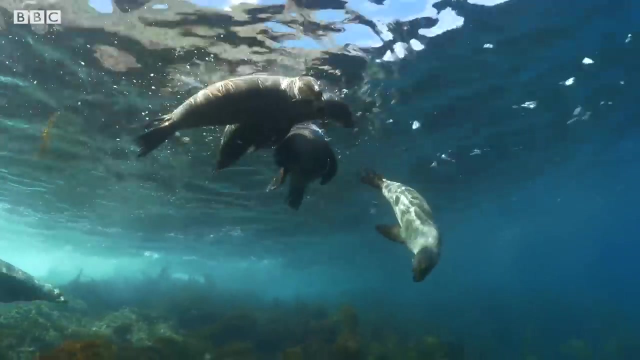 living in an area abundant with food meant their numbers rocketed. The researchers have discovered that female fur seals are being born with a lower birth weight. Only the larger female fur seals are surviving and returning to breed. They're also having their first pups later in life. All this indicates 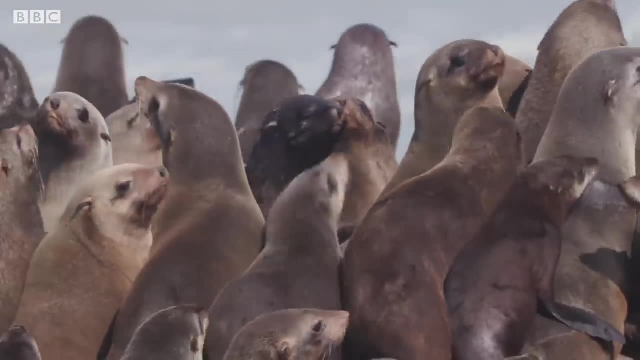 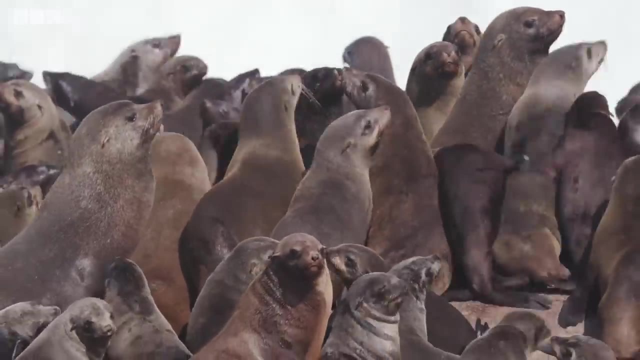 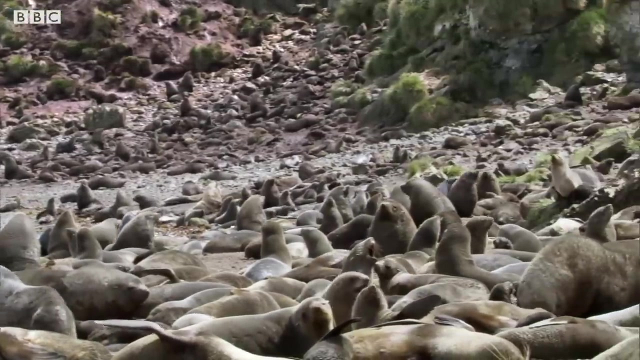 that the females are dealing with food stress. There's just too much competition. These successful females are more likely to have high levels of genetic variation, Which makes them more resilient. The female will seek out a genetically different male to produce stronger offspring When the seals were close to. 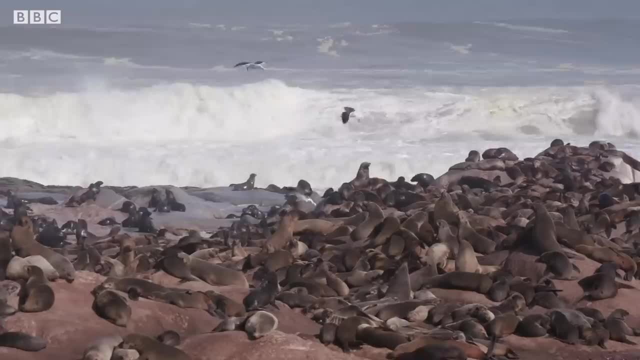 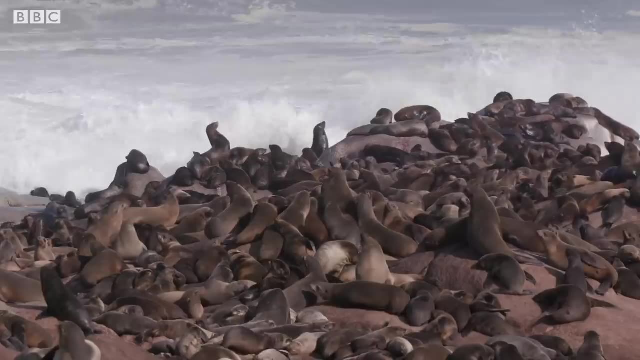 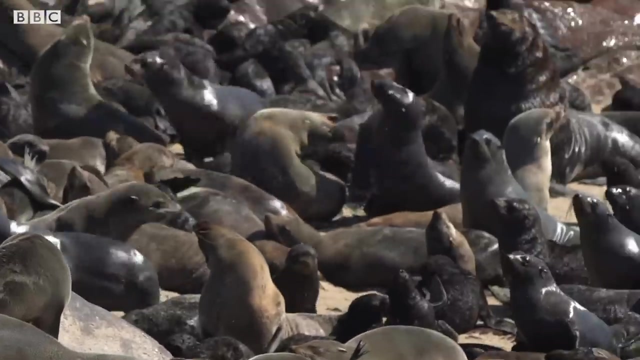 extinction. they faced a genetic bottleneck, But this active choice of a genetically different partner may have helped the fur seal population to explode with such vigor. However, the fact that currently, it's only these super females that are managing to breed demonstrates the stress the population is under. 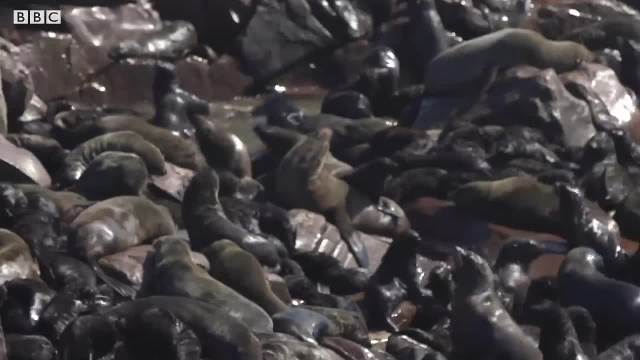 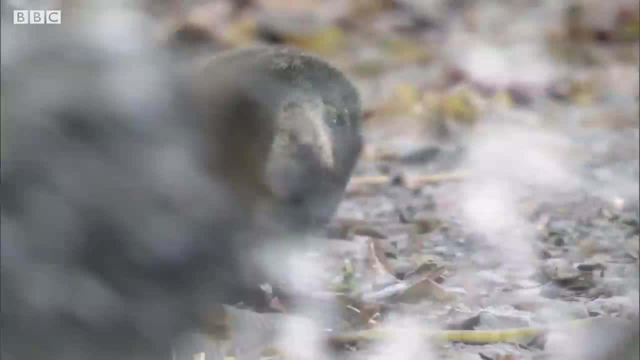 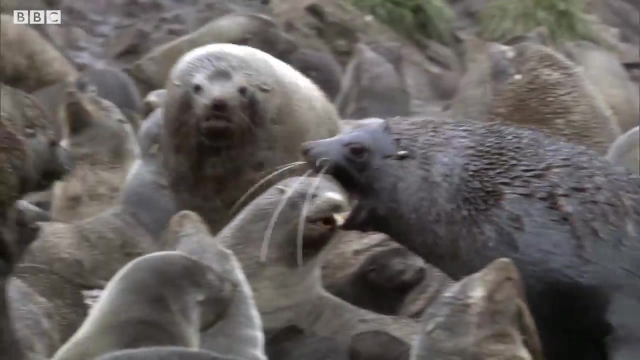 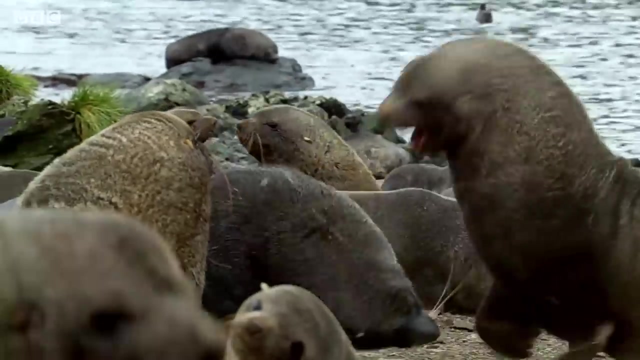 Overcrowding has led to intense competition and stress amongst the seals. Bull seals that weigh on average 126 kilograms and are around two meters in length are territorial and aggressive. Fighting males can often trample fragile pups and severely injure them. Such aggressive behavior from breeding males 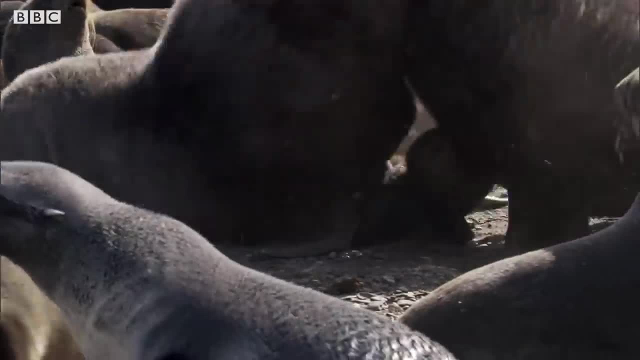 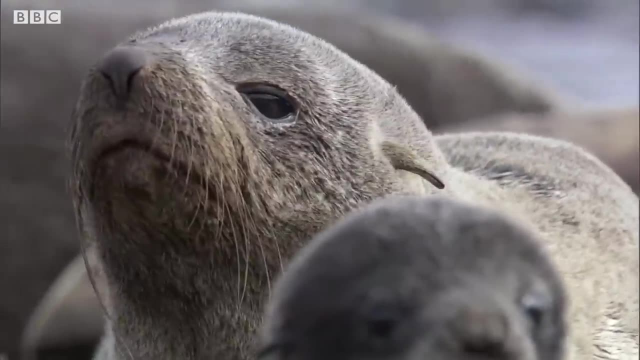 can disrupt mother-pup bonding and lead to pup abandonment. Hungry pups are known to try and feed from any female- A risky move, as females have been seen to attack pups that aren't their own. Starvation and skull injury are more likely to kill. 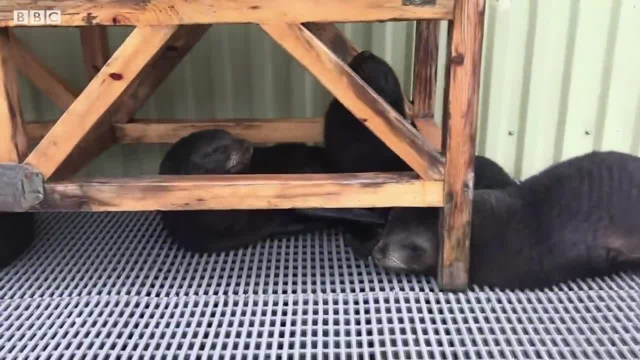 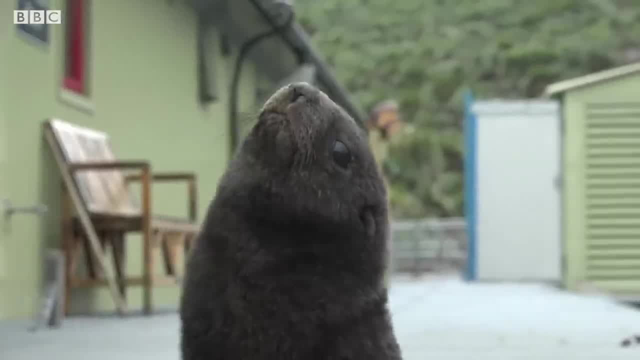 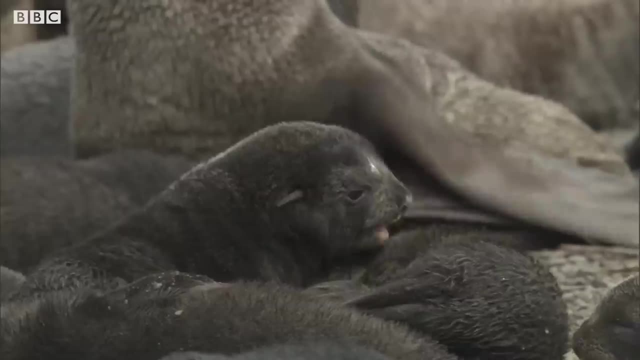 seal pups than anything else. Pups are getting smaller, as food competition means mothers have less milk. We all know stress isn't good, but how is this affecting these young pups? Stress can lead to the production of corticosteroids, increased heart rate and the production of adrenaline. 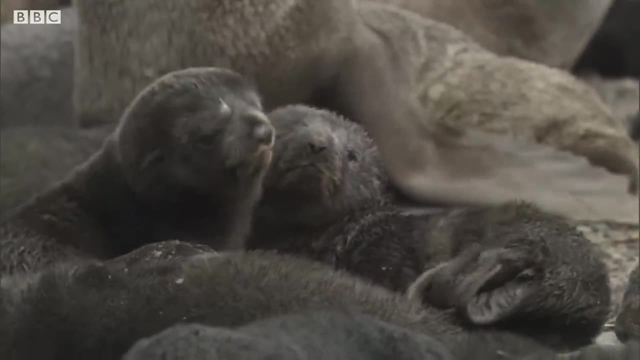 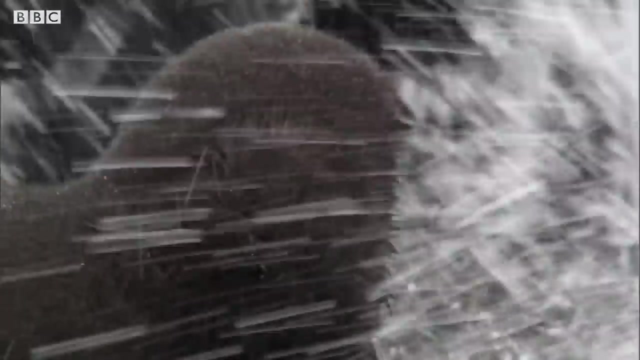 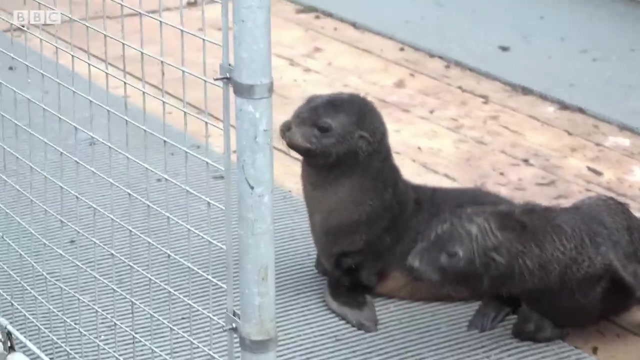 Stress can deplete the energy of a young pup who needs all its reserves to grow and develop. Lack of rest in a calm environment damages their ability to regulate their body temperature and build up the strength they'll need to survive. Stress can even reduce the 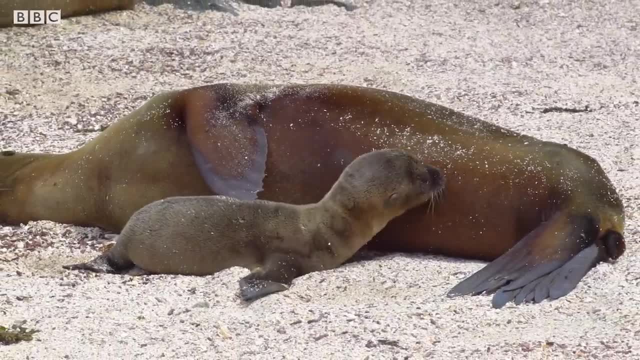 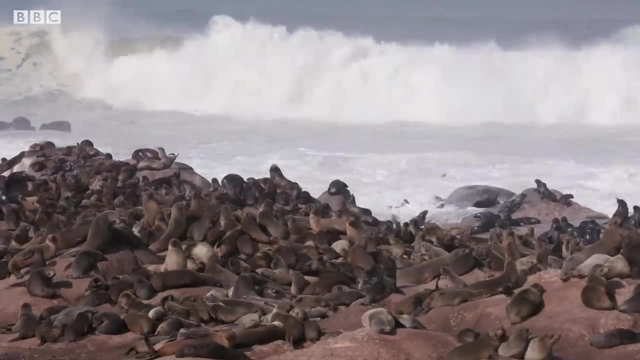 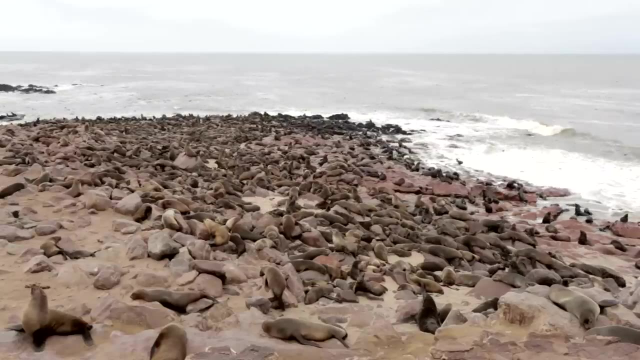 periods of feeding and damage the mother-pup bond. Their time on land is when they build up reserves, so overcrowding and a stressful environment could lead to malnutrition, starvation or death. Overcrowding is not the only challenge facing South Georgia's fur seals: Climate. 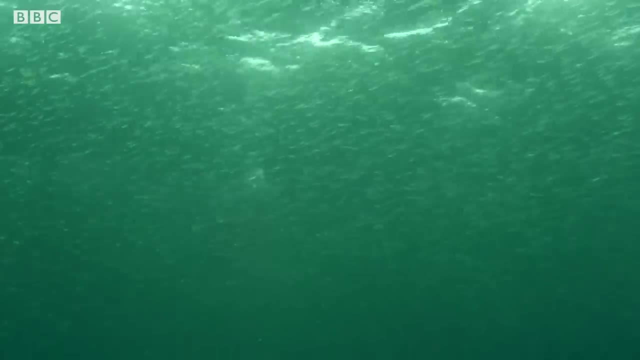 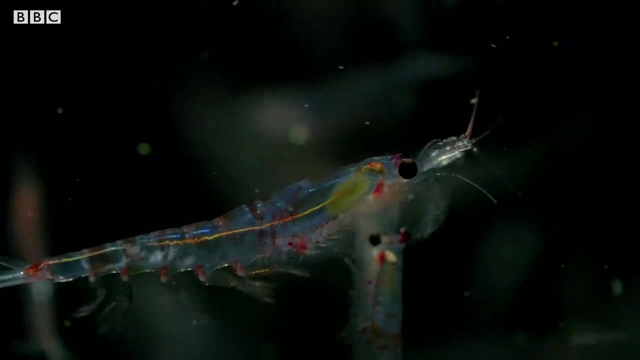 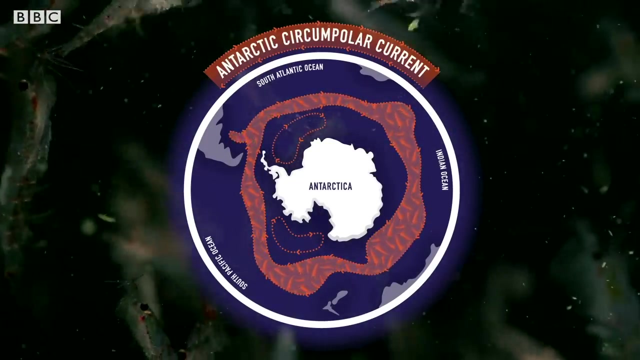 change is also having an impact. Krill forms the majority of Antarctic fur seal diets. The availability of krill is vital in determining the survival of the fur seal population. The Antarctic Circumpolar Current, or ACC, channels nutrient-rich waters towards South Georgia.